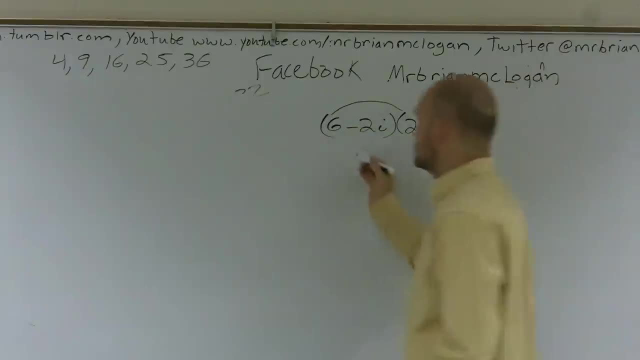 the FOIL method. I'll do my first two terms, which is 6 times 2, which is going to leave me 12.. Then I'll do 6 times negative 3i, which I'm actually just going to write that out. So it's positive 6 times a negative 3i. Then I have a negative 2i times 2, which is minus a 2i times 2.. And then a negative 2i times a negative 2i. 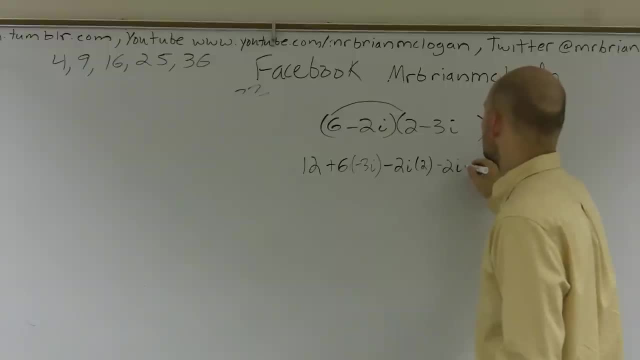 All right. Why do you write it out like that instead of FOILing it? I was FOILing it. I was doing 6 times. Oh, I know, but why did you write it out like that instead of combining them? Because I just wanted to so you could see which multiplications I did, Just stop. Yes, you're right, I was kind of elongating the step. A lot of times I won't go to that step, but I just want to see where you guys 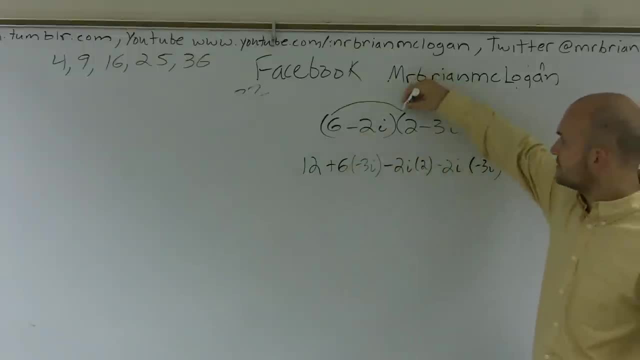 I want you guys to see when I'm multiplying. So I did 6 times 2,, which gave me 12.. I'm sorry I didn't write this out. Then that gives me. well, I did 6 times my 3.. That's my next term. Then I did negative 2 times 2.. And then I did negative 2 times 3i. All right, So we have 12.. 6 times a negative 3i is going to give me a negative 18i. Positive 6 times a negative 3i. This is a negative 2i times 2i. 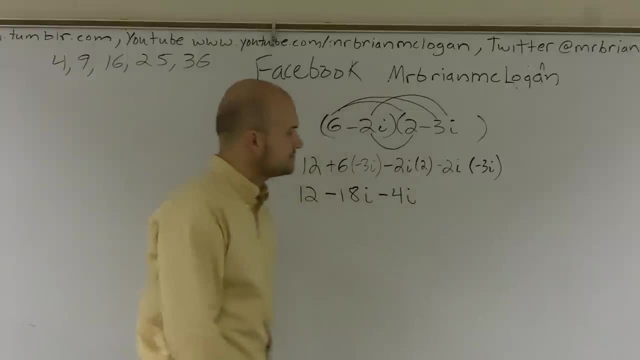 Which will give me a negative 4i, And then a negative 2i times a negative 3 will give me a positive 6.. i times i gives you i squared. And I'm not going to spend a lot of time going into it, but if you guys remember, we like to represent the square root of negative 1, as i, So if I take the square- I'm sorry, I square both of those- I get negative. 1 equals i squared. 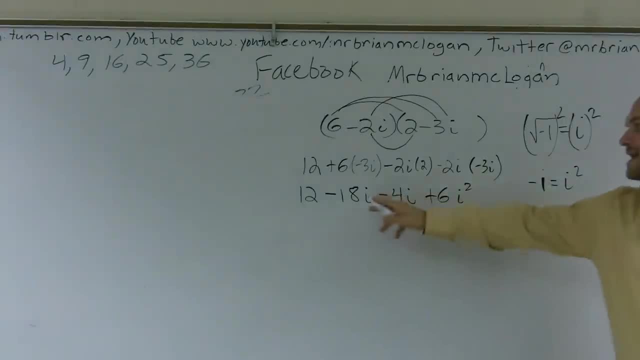 So therefore, I can now rewrite this. I can combine these two terms. Here is where in my i's I can treat them like variables. These are like terms, so I can combine them And I can change this to a negative 1.. So I'm left with 12 minus 22i, plus 6 times negative 1..